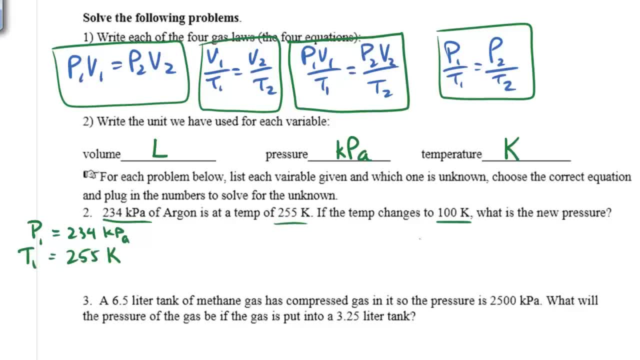 temperature. so that's going to be T2.. And then we don't know the second, pressure. So we've got pressure and temperature, and so what we're going to use is the equation for pressure and temperature. All right, Let's plug everything in. So P1 over T1, 234 over 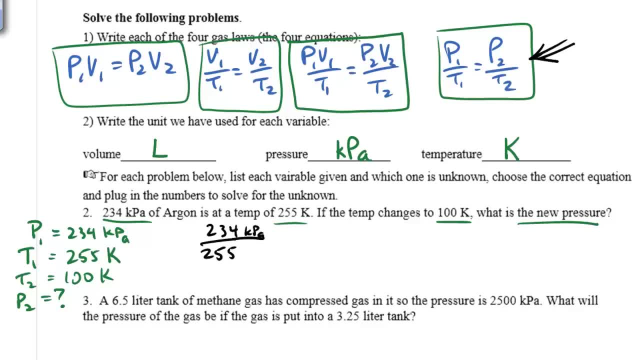 55,, that's kilopascals and Kelvin, And that's going to be equal to P2, which we don't know over T2, which is 100 K. Now, if we multiply both sides by 100 K, the 100 K cancels out. 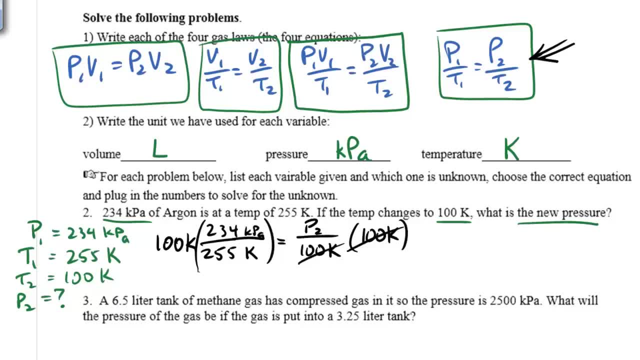 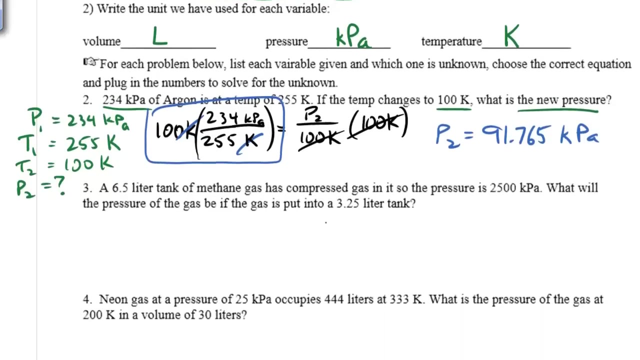 on the right side, leaving P2 equal to this whole thing right here. So P2 is equal to 91.765 kilopascals. Notice, the Kelvin cancels out and you're left with kilopascals. Okay, So all right. We've got liters, so we've got a volume. We've got kilopascals, so a 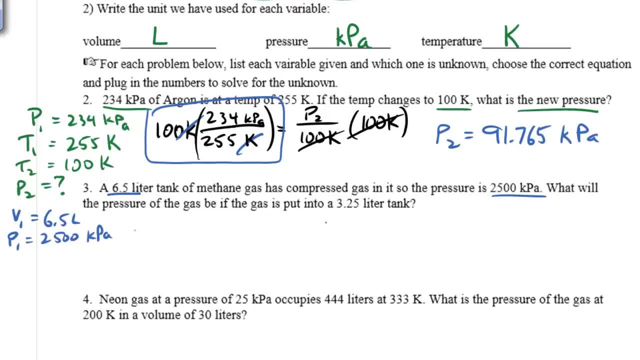 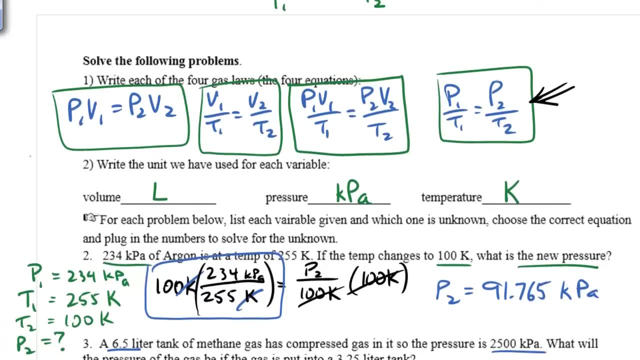 pressure And we've got a second volume, so that's V2, 3.25.. And we don't know P2.. We've got volume and pressure. Gee, I wonder which one we'll reuse. This is the one with volume. 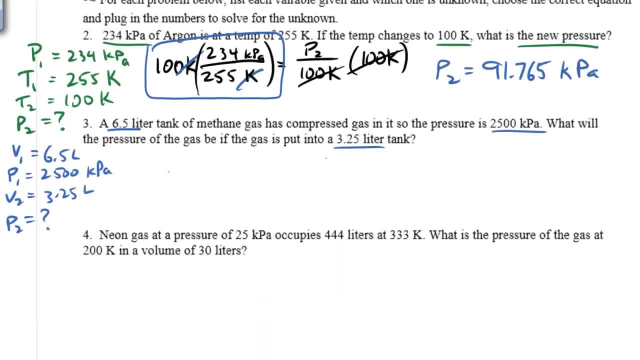 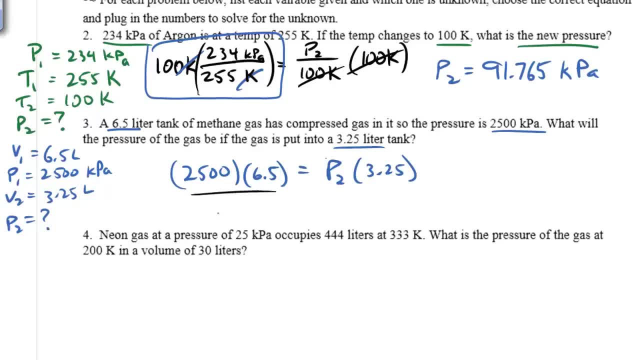 Now, if we go ahead and divide both sides by 3.25, that's going to give us the expression for P2 over here, which equals a grand total of 5,000 kilopascals. All right, next one. 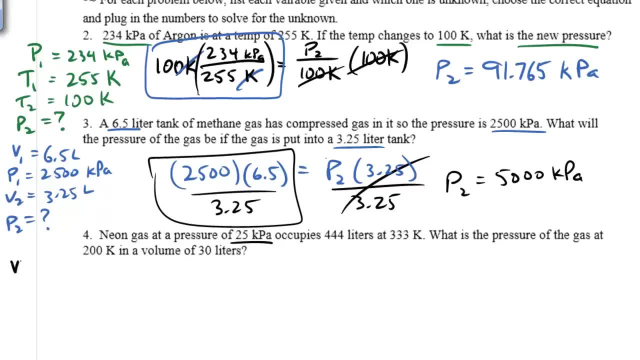 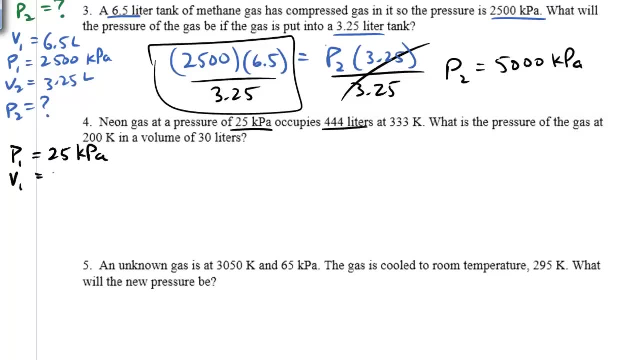 Let's get going here. We've got 25 kilopascals. What is that? Yes, that's right, Not V, but it is P1, and we have 444 liters. That's going to be a volume and a temperature as well. 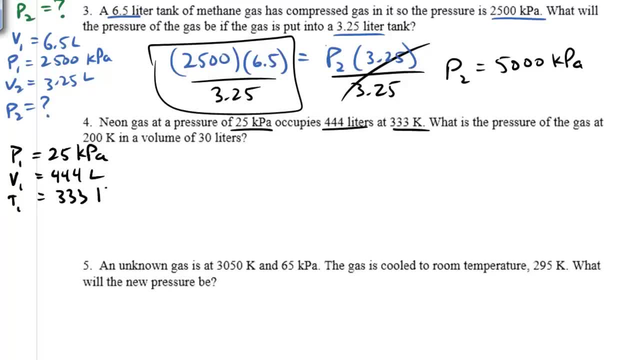 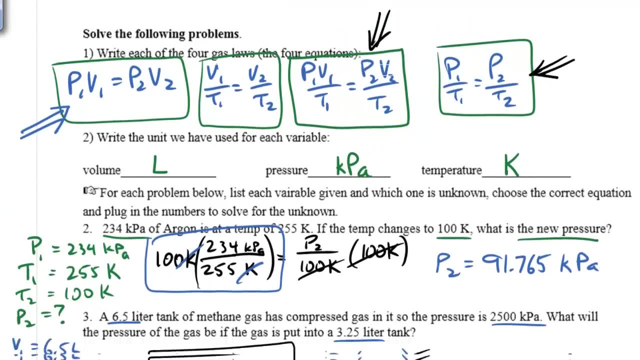 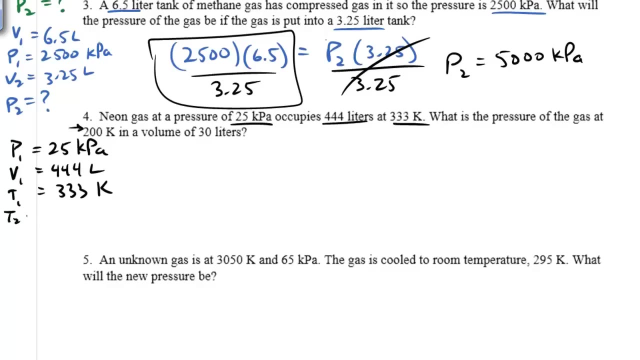 So we know we've got three variables and so we're going to use the combined gas law with all three variables. All right, All right. so what else do we have? We have another temperature, so that's T2, 200 K. 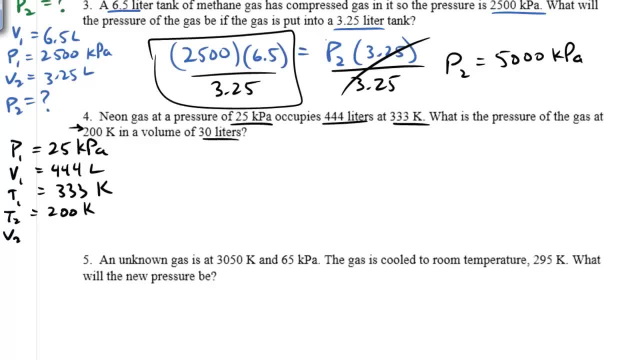 and then finally another volume. We don't know the second pressure, so that's what we're going to find. So P1, V1 over T1, so 25,444.. Over 333 equals P2, we don't know times. V2, 30, over T2, which is 200.. 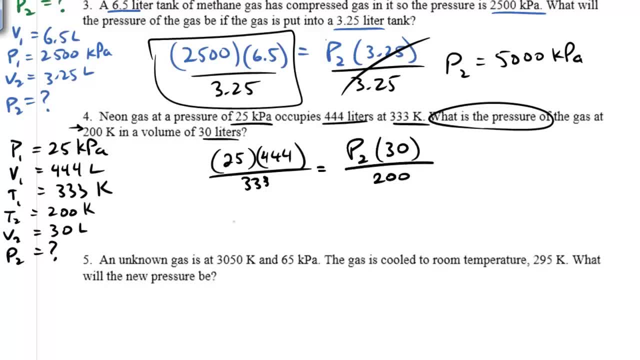 All right. so if we look at what that equals just the left side, it's 33.33, and that is equal to P2 times 30 over 200, or 0.15.. So if we go ahead and divide both sides by 0.15,, 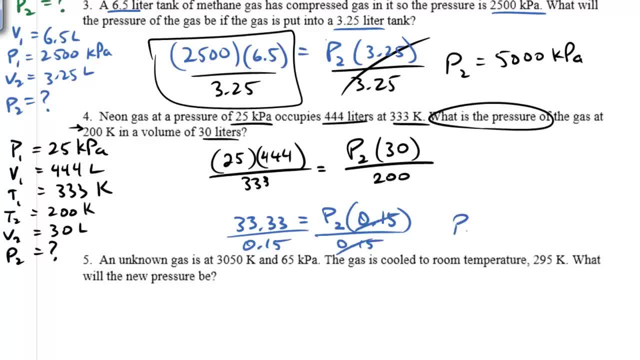 then we have P2 equal to 222.22 kilopascals. All right, Let's just quickly go through the next two. This is a temperature, so that's T1.. This is a pressure, so that's P1..